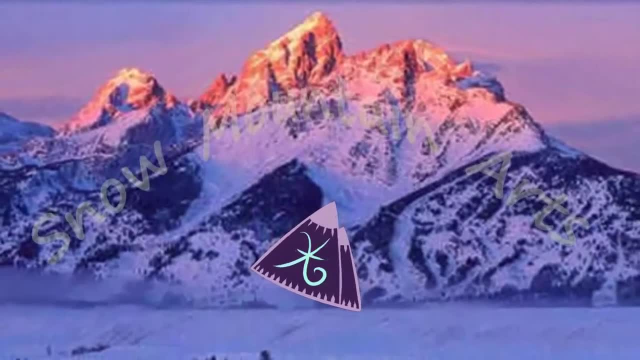 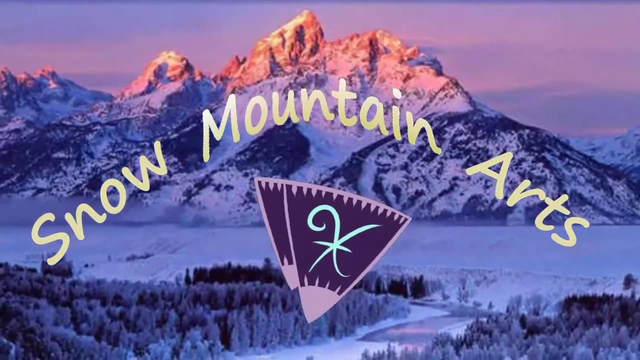 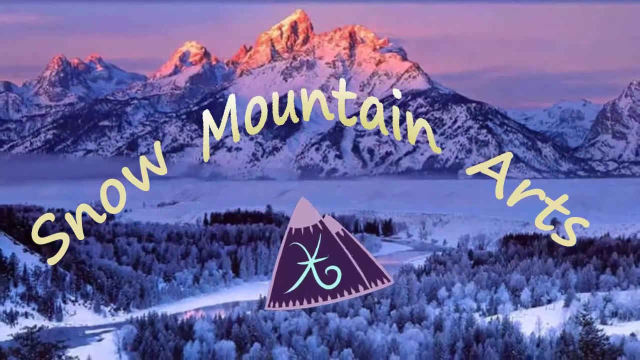 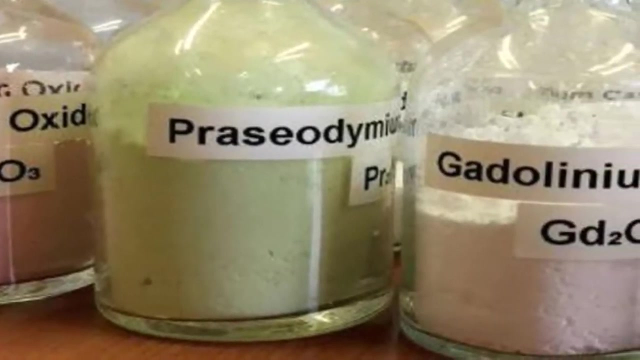 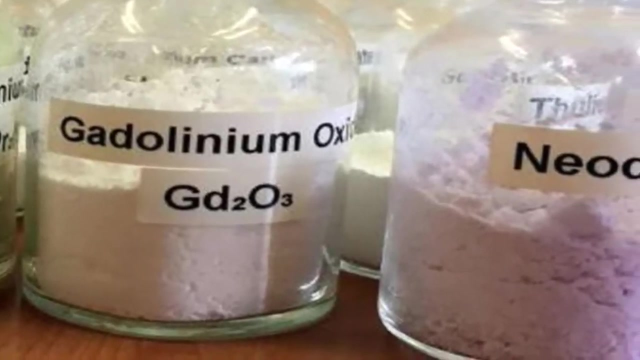 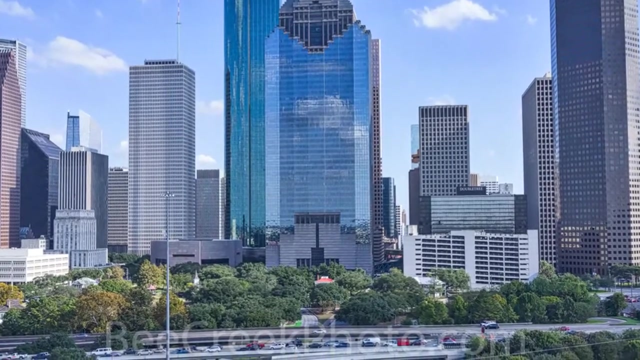 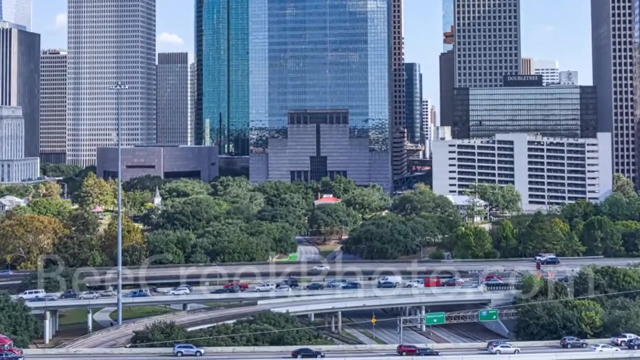 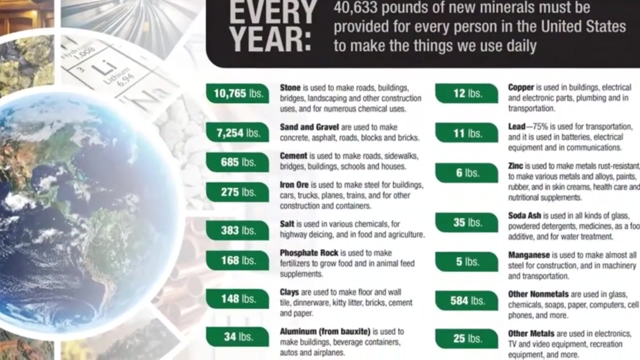 Geology 4.1. Renewable Resources and Non-Renewable Resources. Materials that we extract from Earth are the basis of modern civilization. Mineral and energy resources from the crust are the raw materials from which the products used by society are made. Like most people who live in highly industrialized nations, 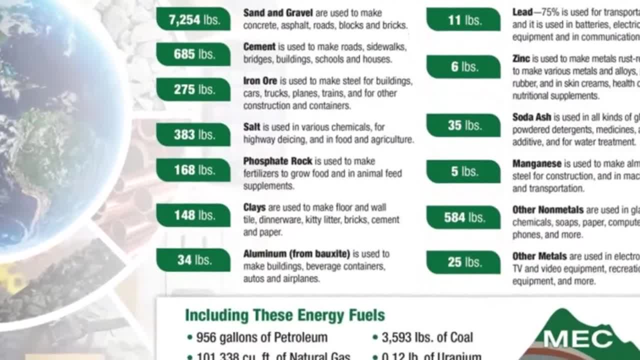 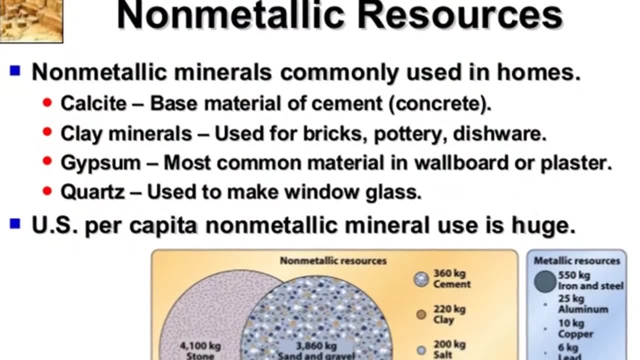 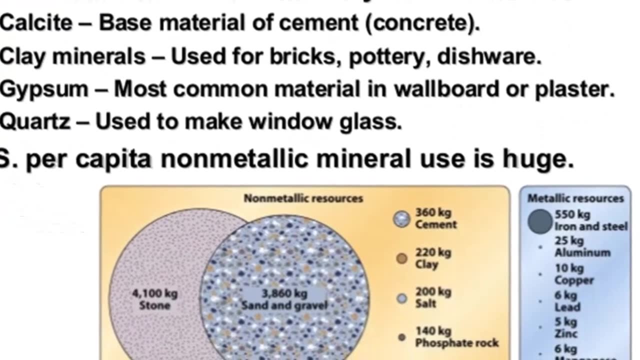 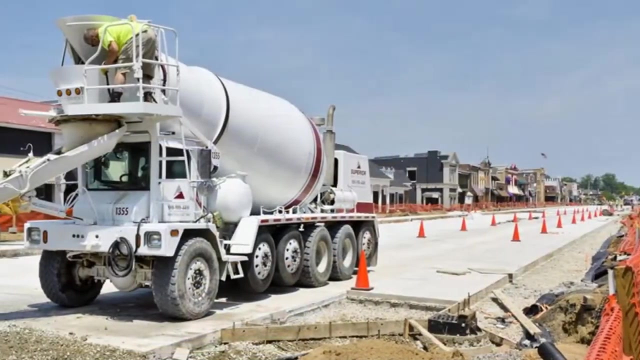 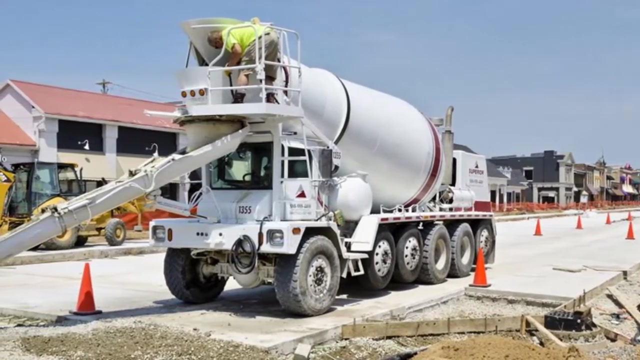 you may not realize the quantity of resources needed to maintain your present standard of living. The annual per capita consumption of several important metallic and non-metallic mineral resources for the United States is each person's prorated share of the materials required by industry to provide the vast array of homes, highways, cars. 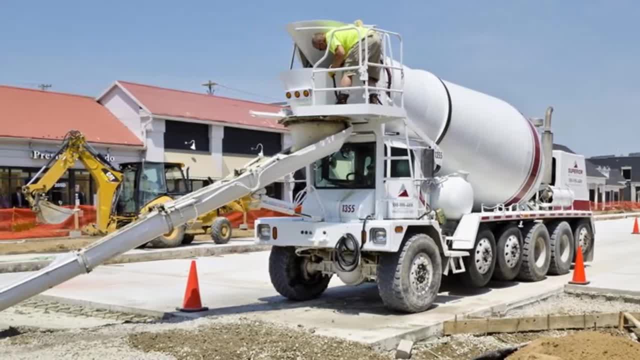 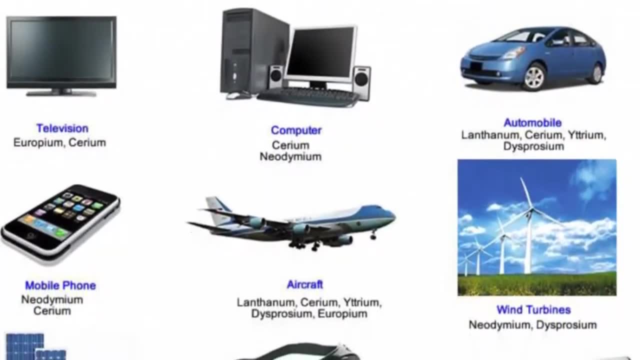 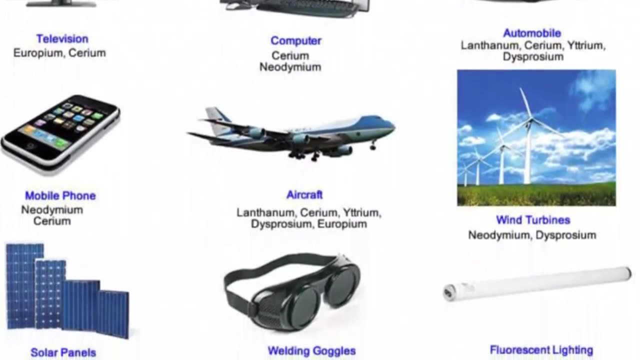 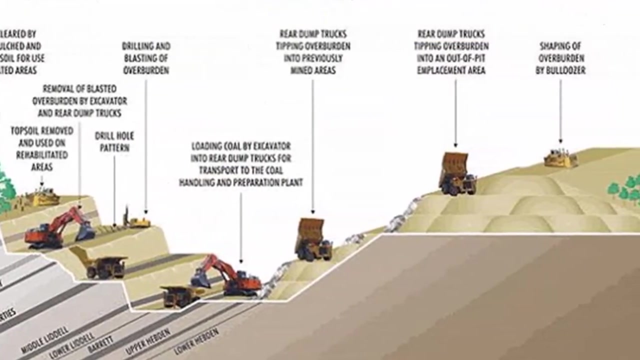 electronics, cosmetics, packaging and so on that modern society demands. The number of different mineral resources required by modern industries is large. Although some countries, including the United States, have substantial deposits of many important minerals, no nation is entirely self-sufficient. 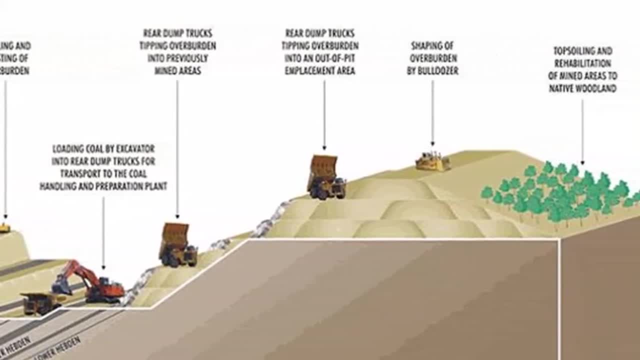 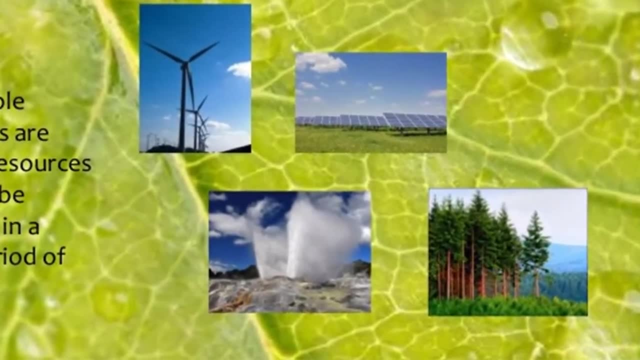 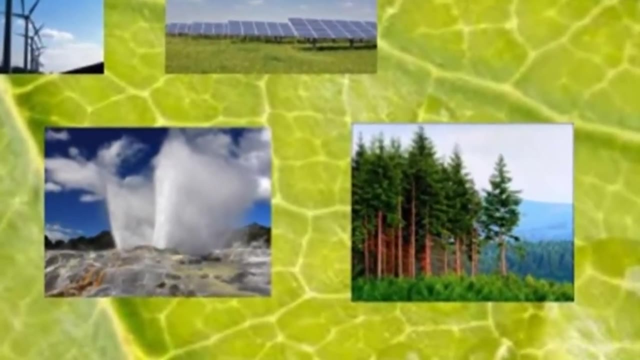 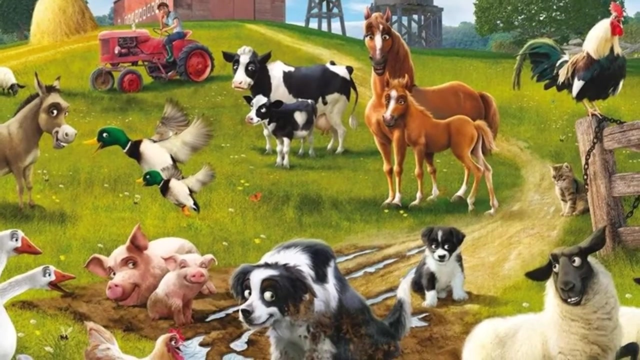 This reflects the fact that important deposits are limited in number and localized in occurrence. All countries must rely on international trade to fulfill at least some of their needs. Resources are commonly divided into two broad categories: renewable and non-renewable. Resources are commonly divided into two broad categories: renewable and non-renewable. 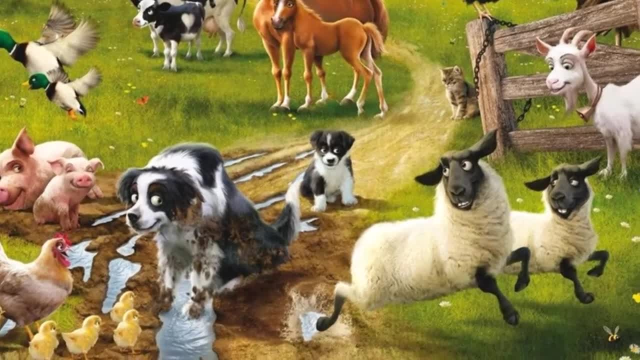 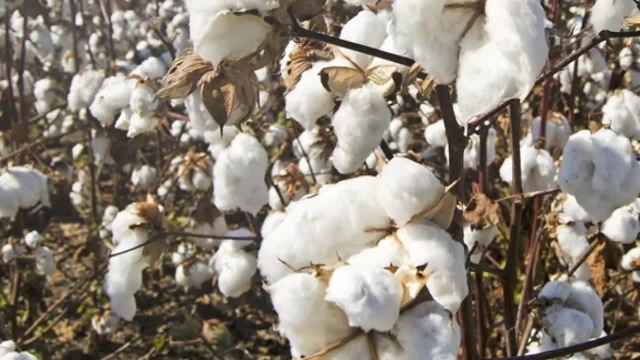 Resources are commonly divided into two broad categories: renewable and non-renewable. Renewable resources can be replenished over relatively short time spans, such as months, years or even decades. Common examples are plants and animals for food, natural fibers for clothing.